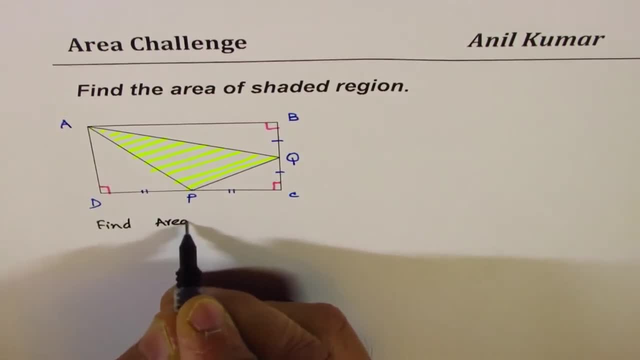 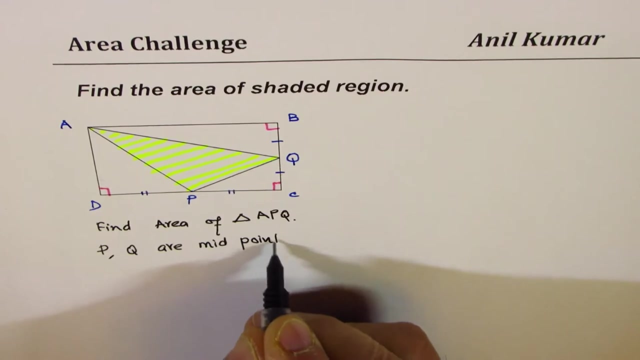 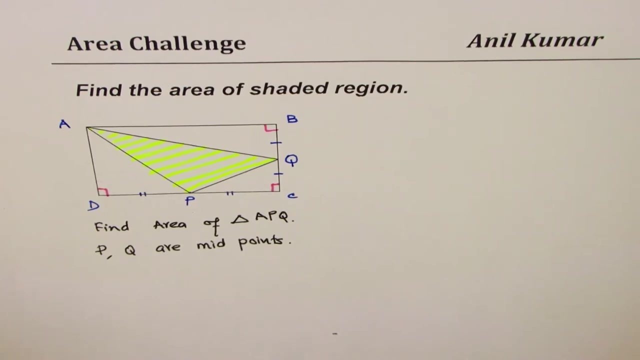 area of triangle A, B, Q. okay, And, as you can see, P and Q are midpoints. P- Q are midpoints. Perfect, You can always pause the video, answer the question And then look into my suggestions. So in general, let's say the side lengths are X and Y. 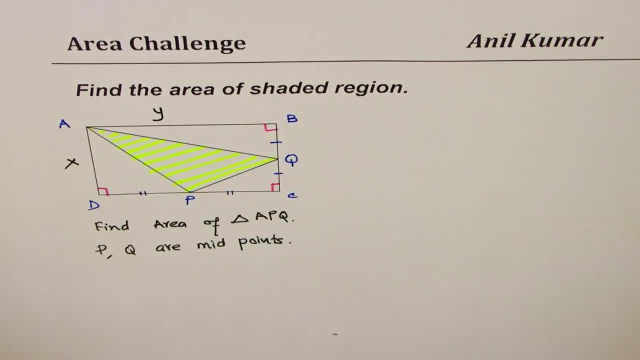 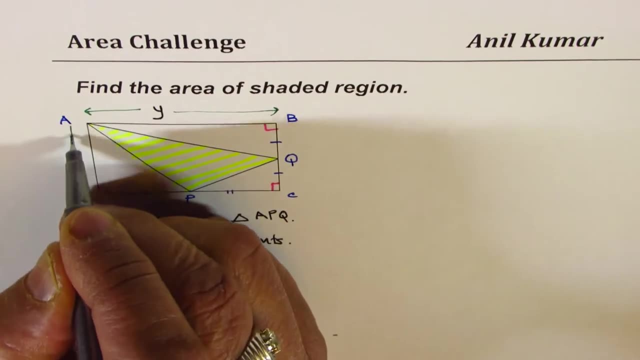 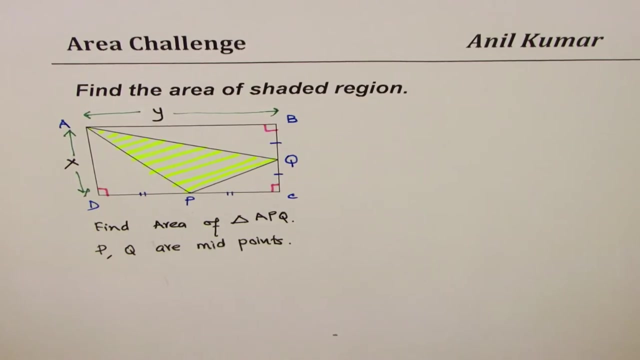 So we'll put this length as X and this as Y, Is it okay? So we're just taking our dimensions X and Y for our rectangle so that we can work with some, some variable values and get to the result. I hope now the question is absolutely clear. You can pause the video. answer the question. 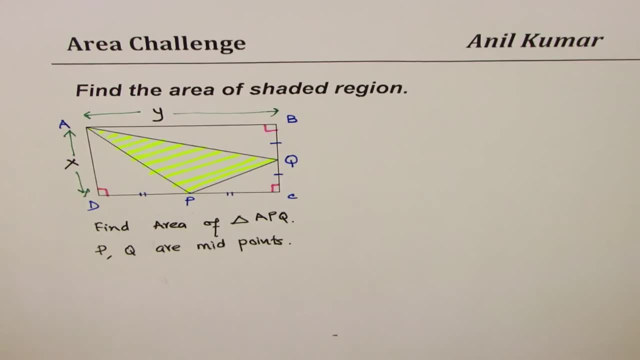 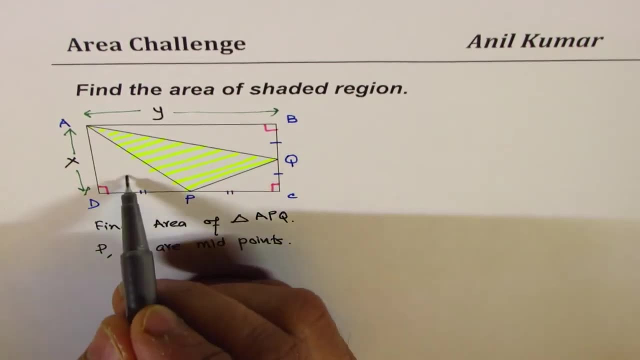 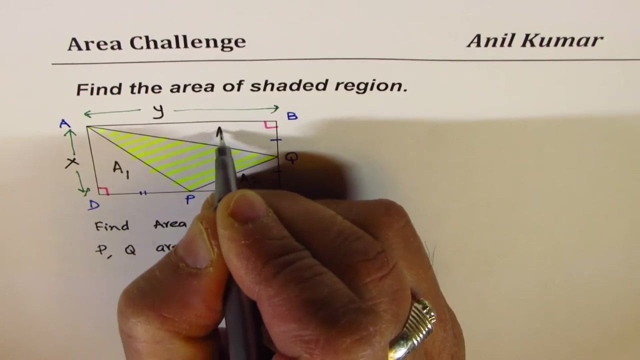 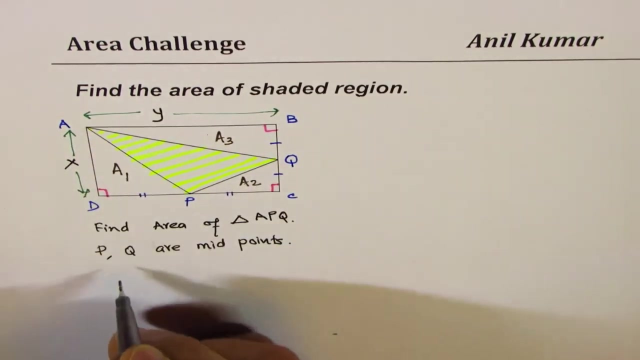 and then look into my suggestions. Well, the strategy here is to find the area of triangle will take away area of these small triangles from rectangle. So let's call these small triangles as A1, A2 and A3. right Now, what is the triangle of? what is the area of rectangle? 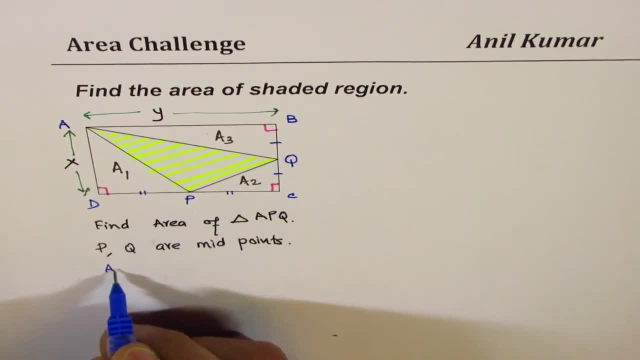 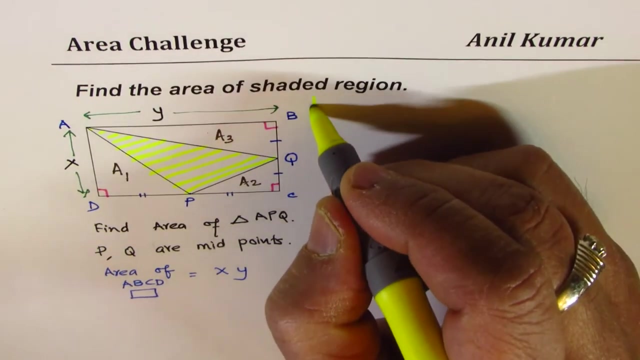 Okay, it's base into height, correct? So let's write down area of a, b, c, d, which is a rectangle. right is clearly x times y, no doubt about it, correct? so that is the total area from where we are going to subtract area of these three triangles. 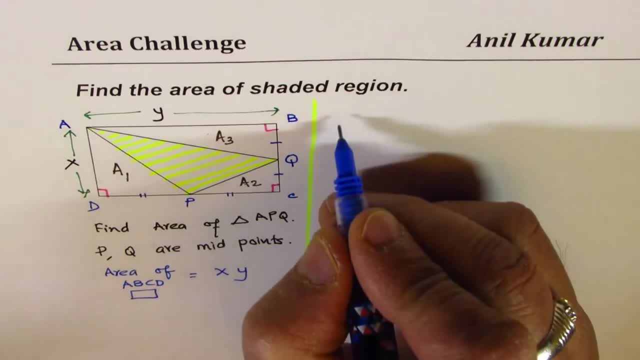 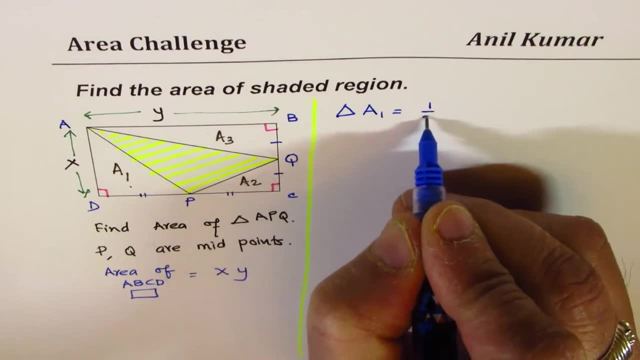 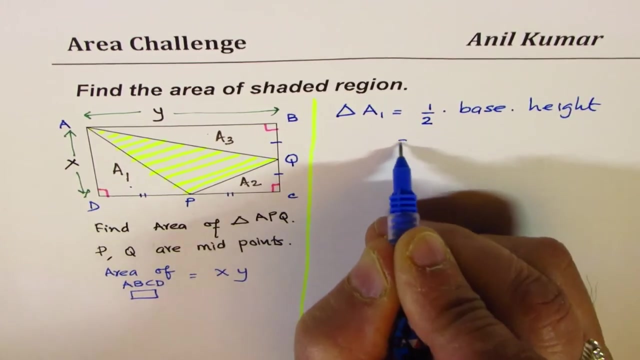 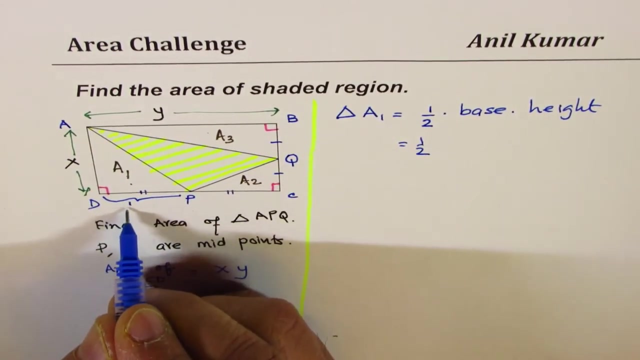 so let's consider them one by one. so what is the area of triangle a1, a1, this triangle area of the triangle formula is half base times height. so in this case it would be half. and what is base? how much is this? this is half of y, right? this is half of y, is it okay? so base is half y. 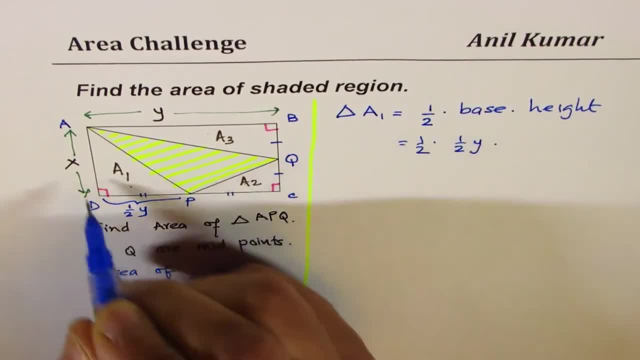 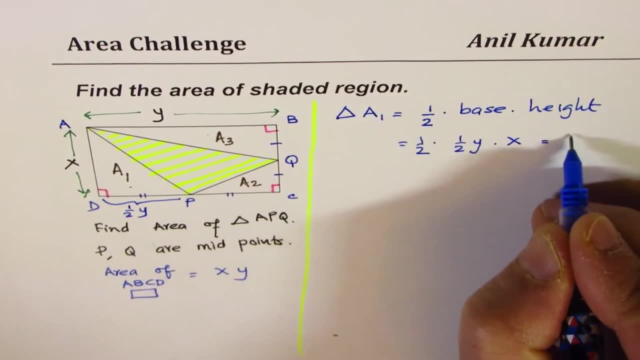 so base is half of y and what is the height? height is x for us. okay, so that becomes the area of triangle. triangle 1, I could write this as 1, 4th of x, y, Perfect. What is the area of triangle A2? This: 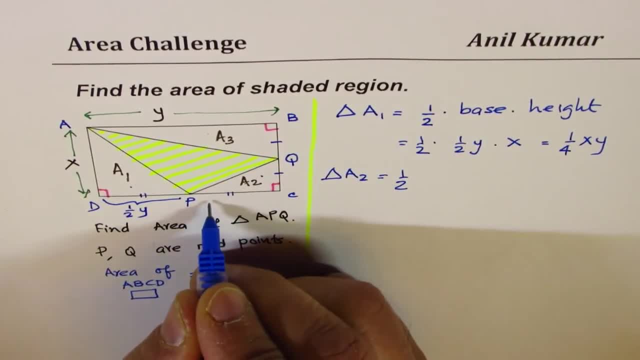 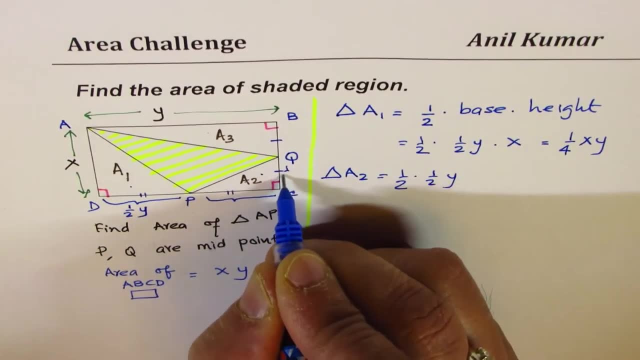 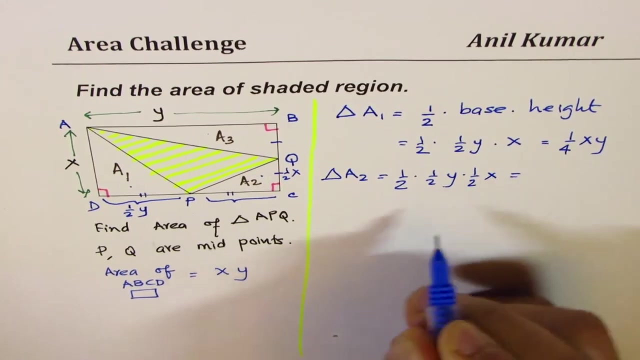 triangle, Again: half Base. base is how much. This is my base. Half y right. Half y times this is half x. correct Total is x, half of it. So half times x. That gives us how much. 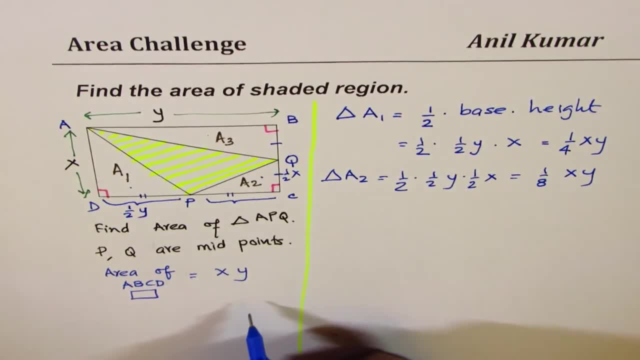 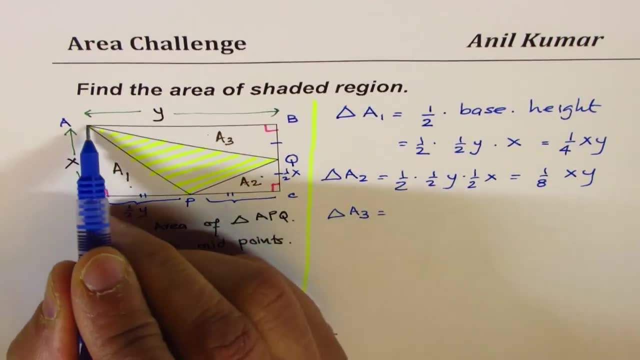 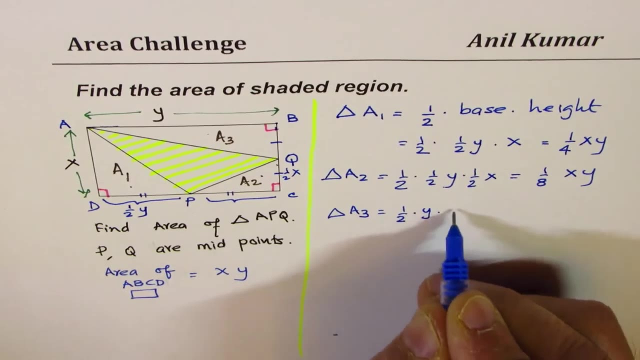 1 over 8, x, y. Now let's consider the triangle A3. In this triangle, base is y and height is half of x. So the area is half times y times half of x. That gives us 1 4th of x. 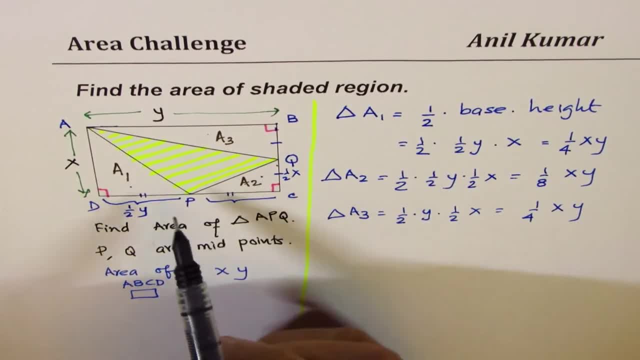 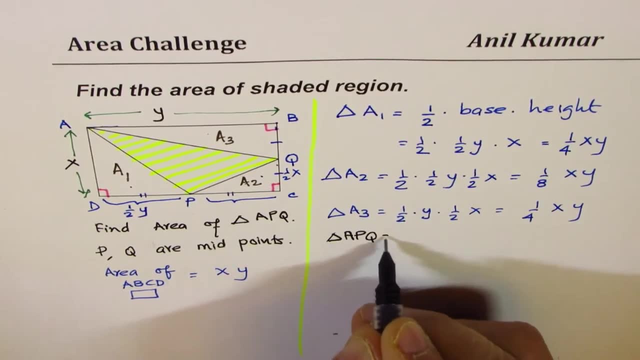 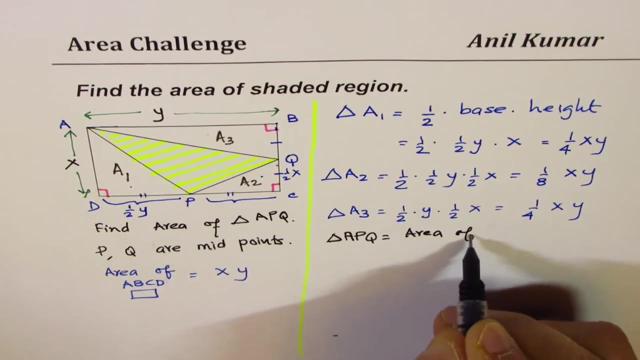 y. Perfect. Now to find the area of APQ triangle, let's write down triangle A3.. So A, B, Q, It should be area of rectangle right. Area of rectangle A, B, C, D. Take. 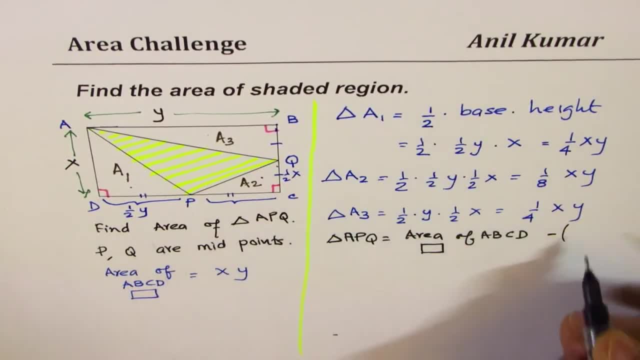 away A1,, A2, A3, right. So take away area of triangles A1, A2, and A3.. So take away A3, correct? This is what it is. So let's rewrite Area of rectangle as we know is. 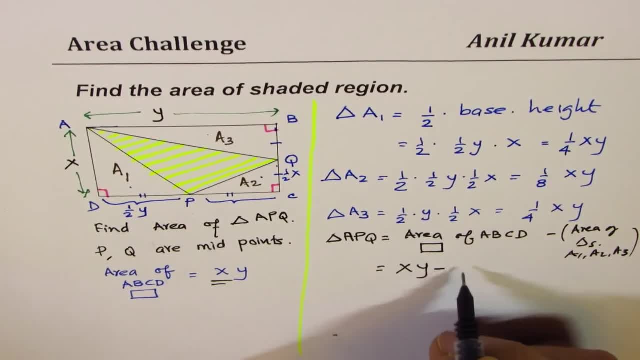 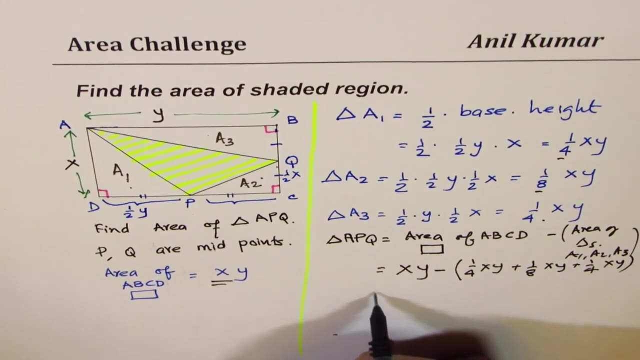 x y. Perfect, This is what Minus we'll add all these. So we'll add these things: Minus 1 4th of x y plus 1 8th of x y plus 1 4th of x y. Okay, So it means x y minus. 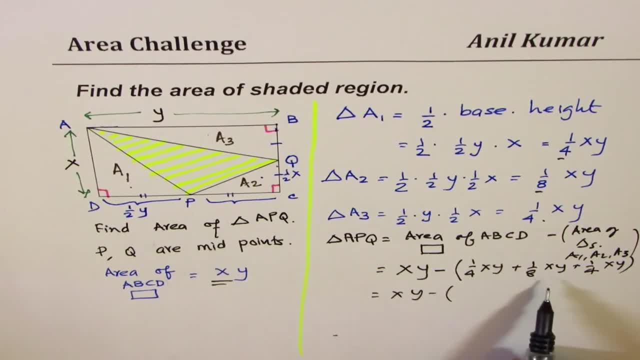 how much. So all this? you can take 8 as your common denominator, right? So 8 is your common denominator, Let's say 8.. Then you get 2 x y plus x y plus 2 x y. So that gives you x y minus 2,, 3,, 4,, 5.. 5 x y over 8.. So it is 8 x y minus 5 x y.